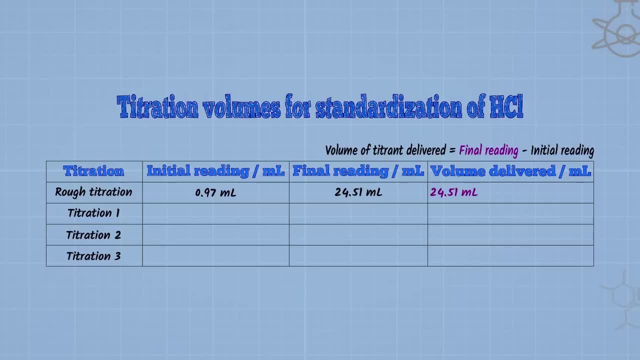 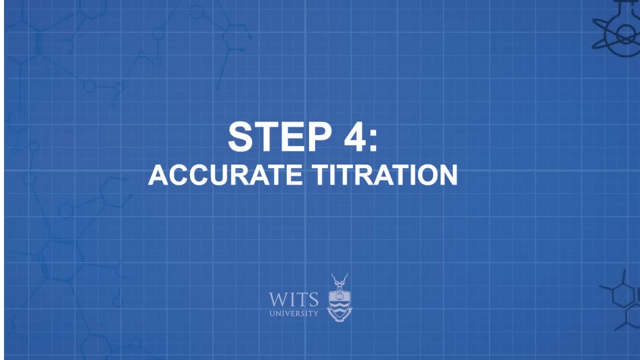 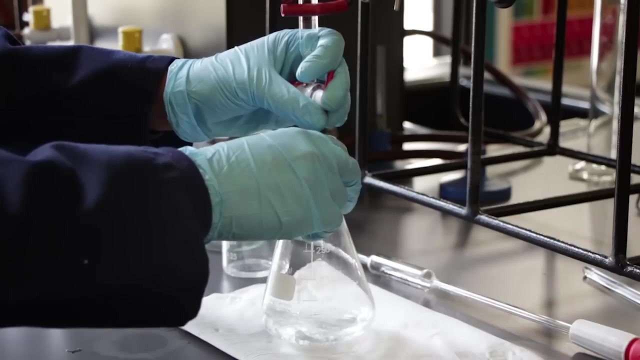 is determined by subtracting the number of drops of the indicator. The number of drops is the final reading. with the initial reading, The burette will then be refilled, Initial readings recorded and the solution in the conical flask prepared in preparation for the next titration. The next titration will be done carefully to ensure that the endpoint 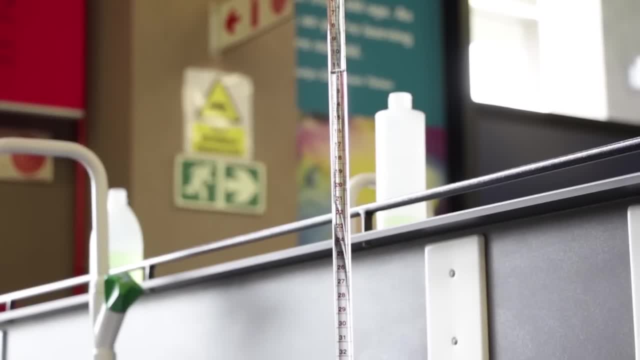 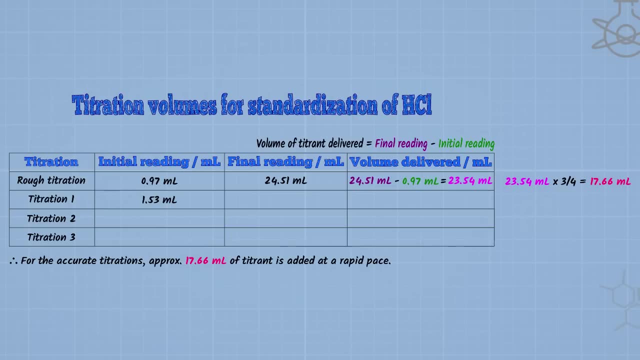 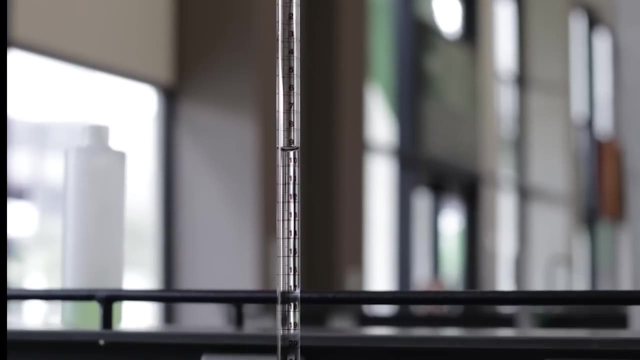 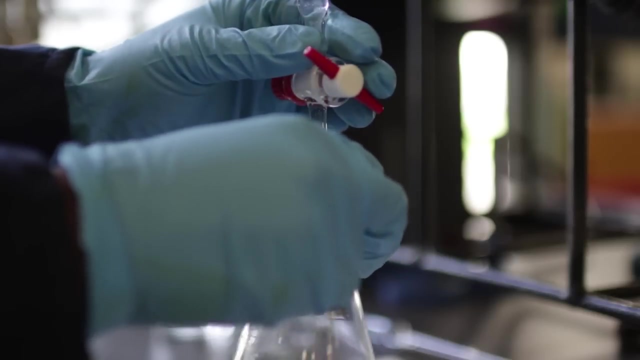 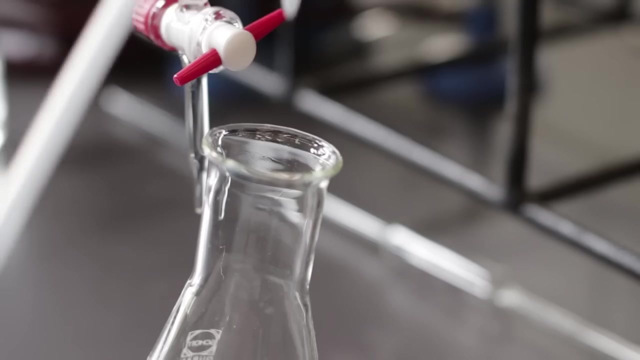 is not missed. using the volume recorded during the rough titration, The general procedure is to deliver the following results: It is even possible to add a drop, swirl, add another drop, and so on until an endpoint is reached. When approaching the endpoint volume, a good habit is to wash the sides. 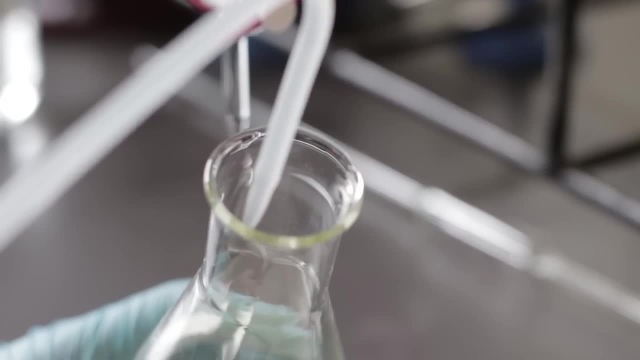 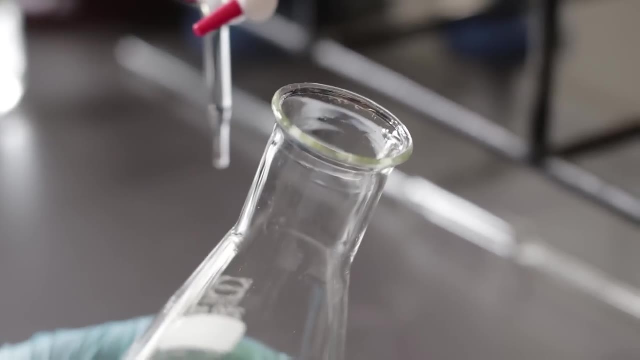 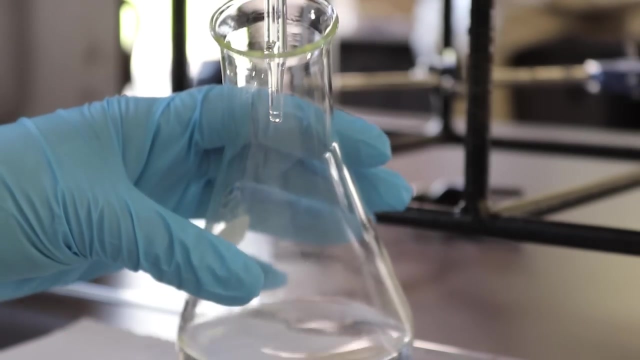 of the conical flask with distilled water from a wash bottle, As when swirling, the side of the conical flask will touch the tip and some of the titrant will stick to the walls of the flask If there is a droplet hanging on the tip of the burette. 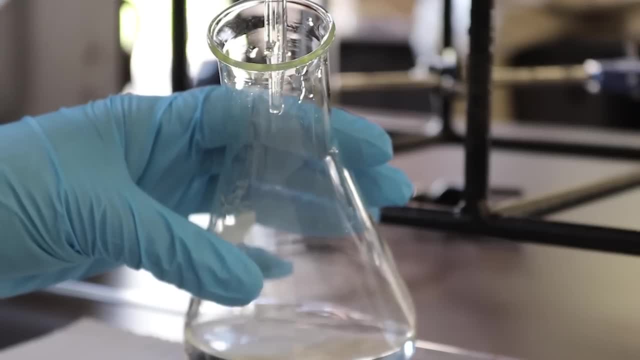 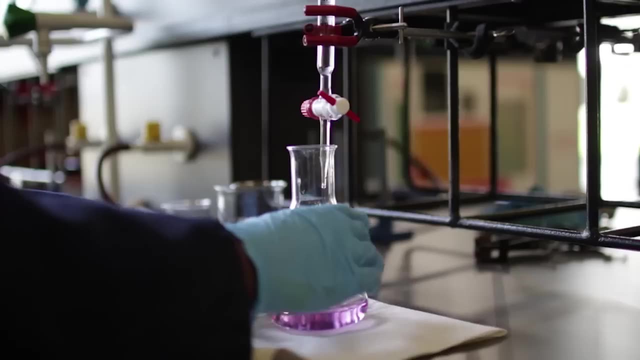 wash the droplet into the flask using a wash bottle, especially when approaching the endpoint. Washing off the titrant will result in a more accurate and precise result. Once the endpoint is reached, the final reading will be completed. The final reading will be completed and the 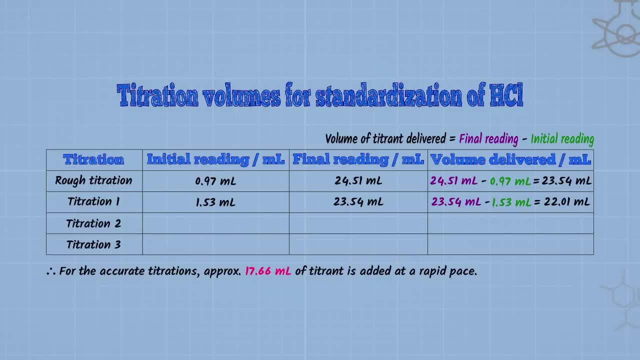 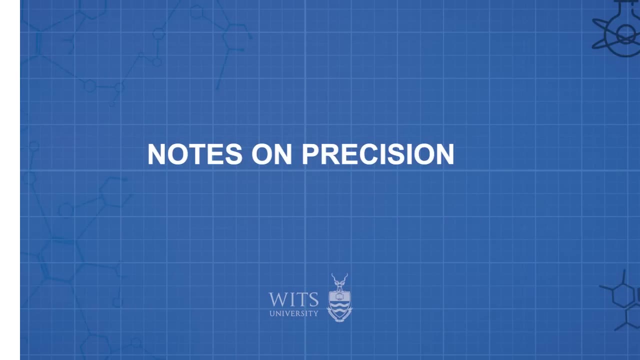 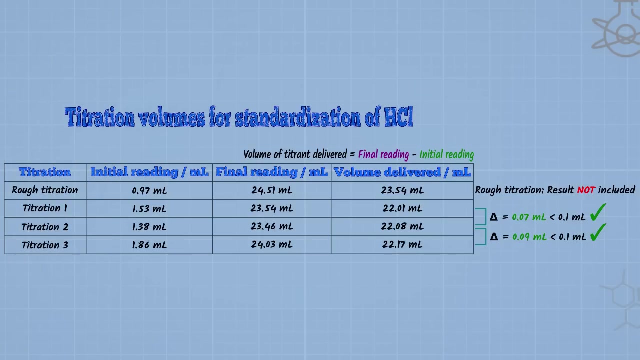 final reading is taken and the total volume of titrant delivered is determined by subtracting the final reading from the initial reading. Titrations are generally done in triplicate, so you will need to perform two more titrations To get precise results. your volume of titrant delivered for the three non-rough titrations: 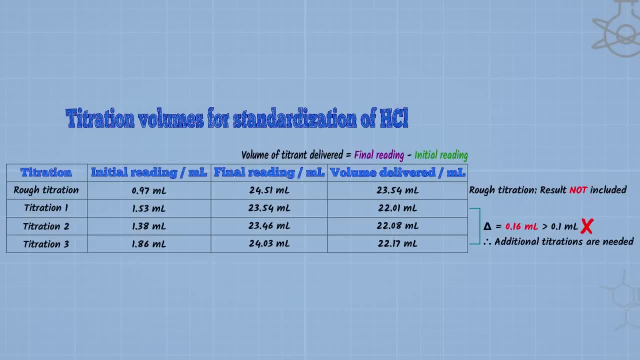 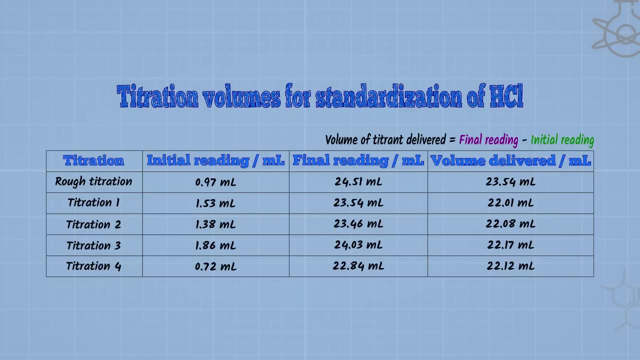 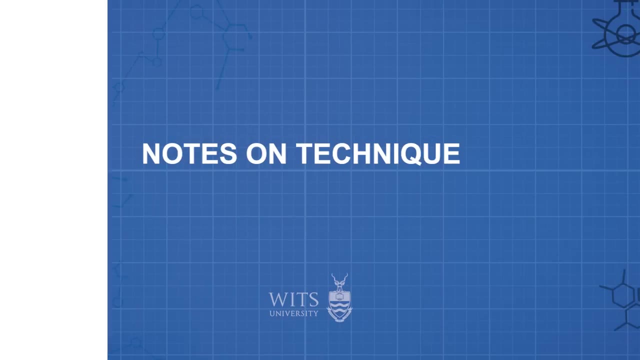 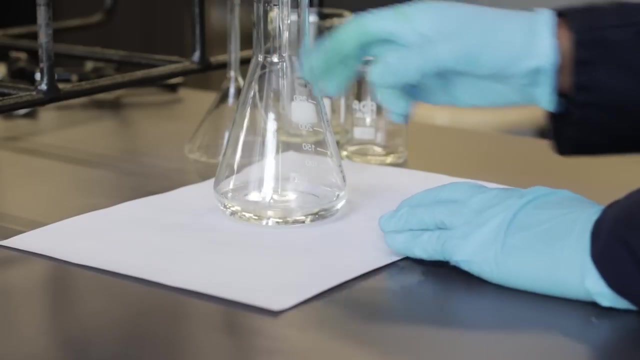 should be 0.1 mL. difference between 0.1 mL and 0.1 mL. If this is not the case, additional titrations will be performed to get precise results. To better observe the colour change of the indicator, a plain white piece of paper is. 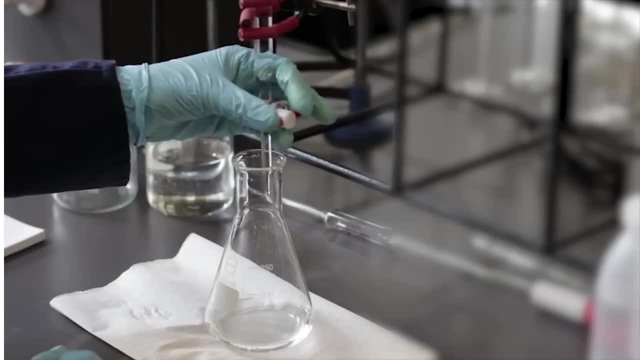 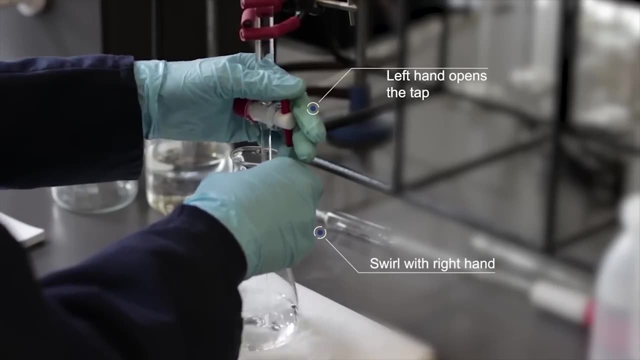 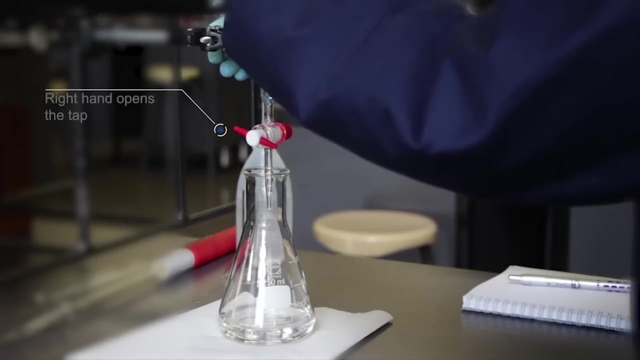 placed under the conical flask. For right-handed individuals, the burette tap will be handled using your left hand, while the flask is swirled with the right hand. However, for left-handed individuals, the burette tap is handled with the right hand and the flask swirled using 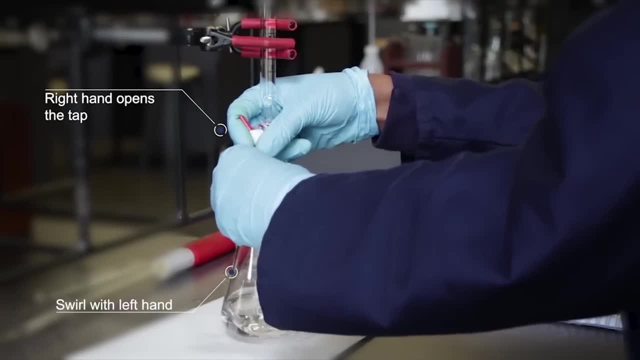 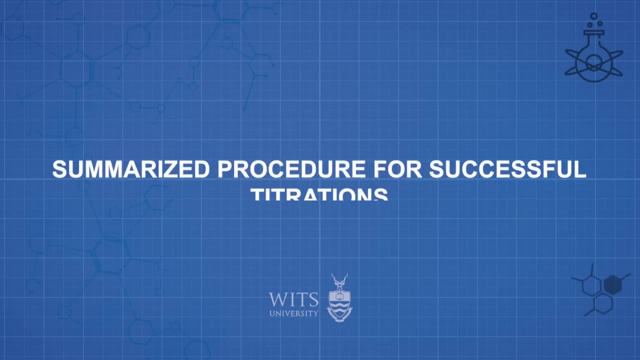 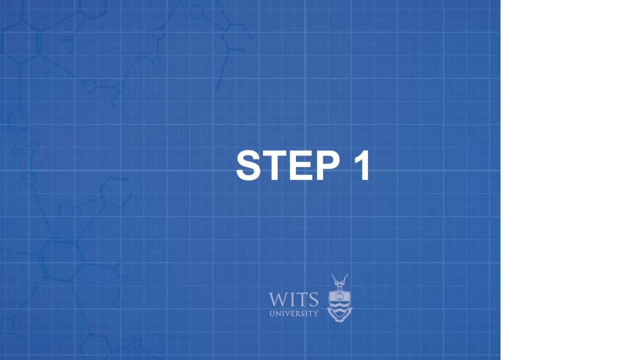 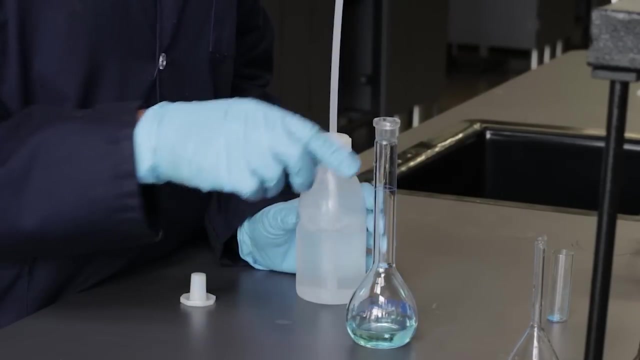 the left hand. In this case, the left-handed individuals will have to reverse the burette to accommodate their titrations. Here is the summarised procedure required for successful titration: Step 1. If the sample is a solid, it is weighed and then dissolved to make up a known volume. 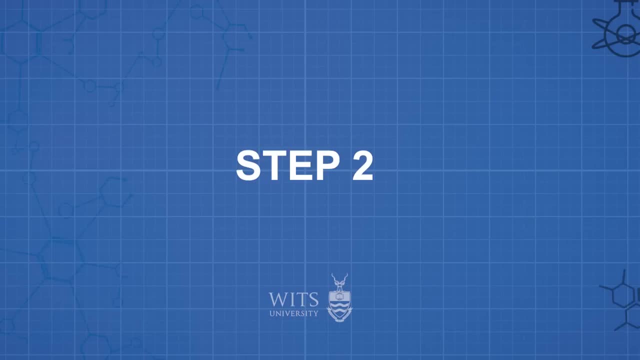 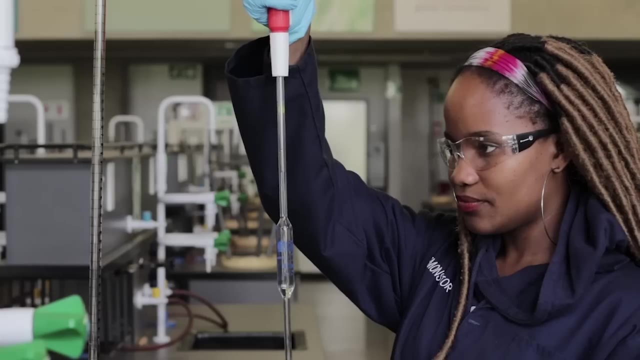 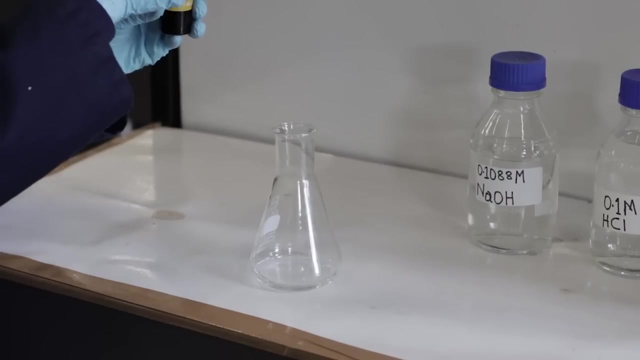 of solution in a volumetric flask- Step 2.. A pipette is used to measure accurately a volume of this solution, for example, 10.00 mL. This is emptied into a conical flask- Step 3.. A few drops of an indicator may be added to the conical flask. 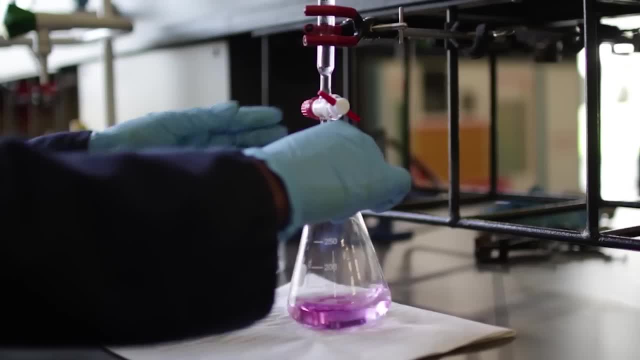 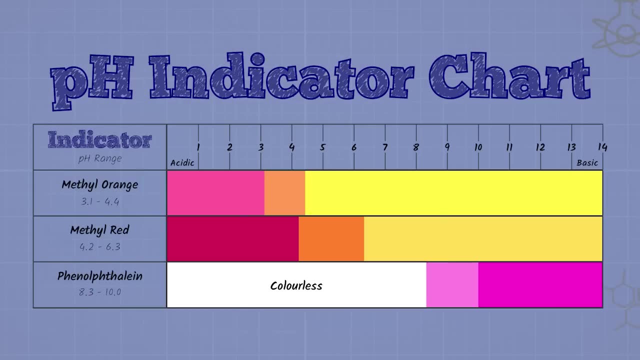 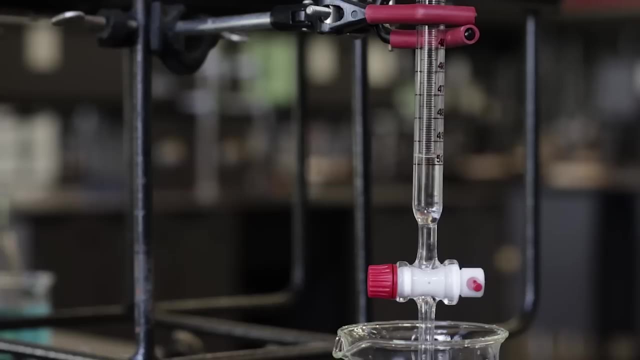 This will show a change of colour once we have reached the end point or when the titration is complete. The following indicators will be used in your practicals: Step 4.. A second solution is placed in a burette. This is the titrant This solution contains. 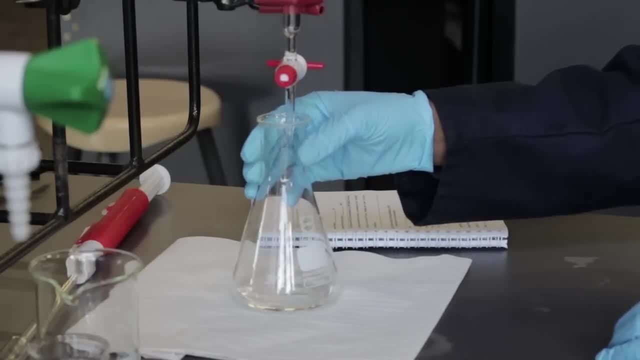 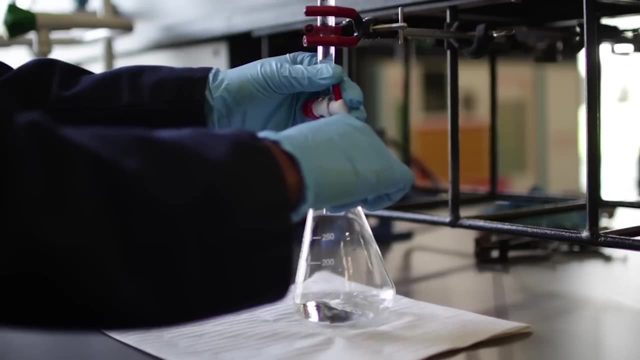 a chemical that will react with the analyte chemical sample in the conical flask, Step 5.. The solution from the burette is run into the conical flask. The solution is added one drop at a time and swirled to mix the solutions as the end point. 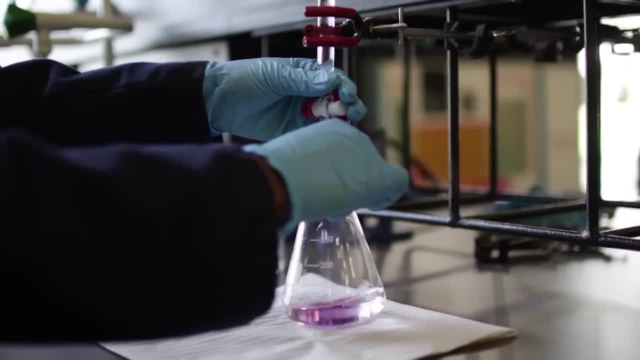 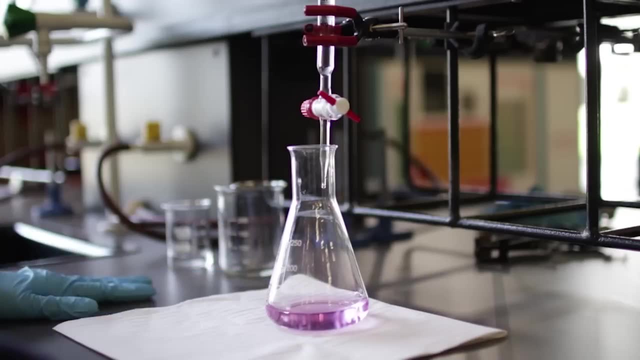 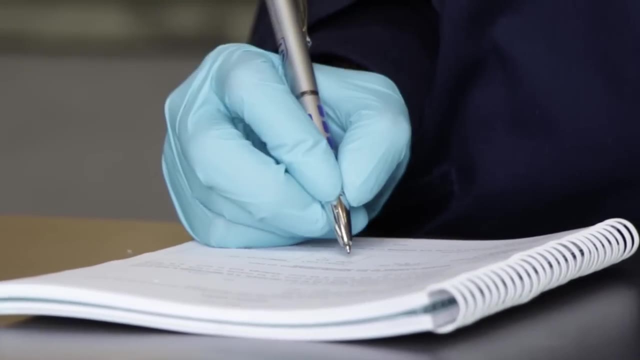 is approached Eventually. a colour change shows the correct amount that has been added to react completely with the analyte chemical in the sample, Step 6.. The volume of solution added from the burette is noted. The titration results can then be used to calculate concentration. Using the following steps ensures that your 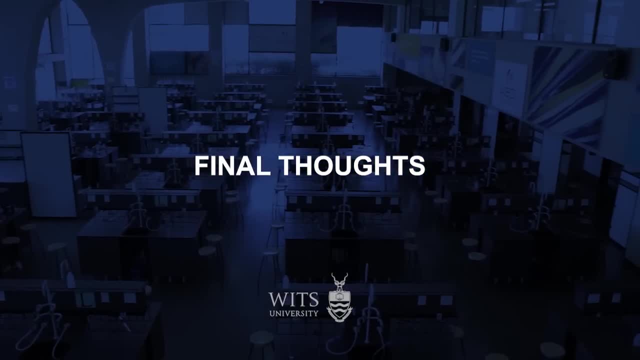 titration experiments are carried out using the correct techniques that enable you to get precise and accurate results.